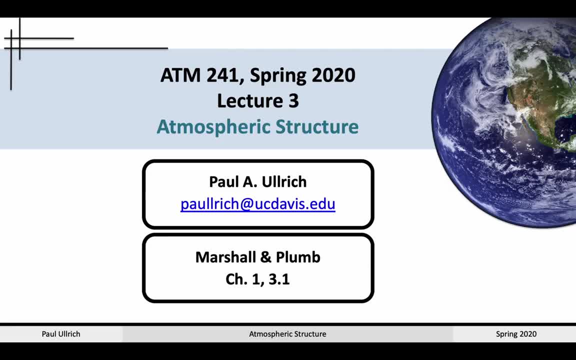 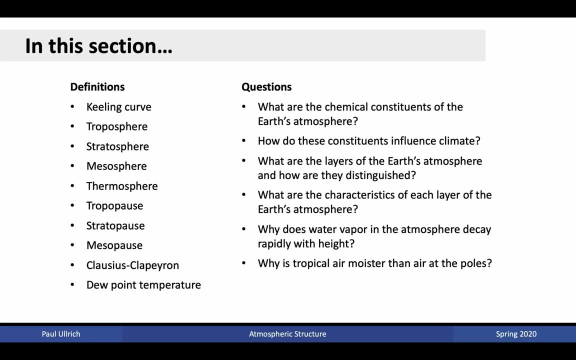 Hello all. welcome back to Climate Dynamics. Today we're going to be talking about atmospheric structure, in particular, focusing on the vertical structure of the atmosphere. The reference reading for this is Marshall and Plum, chapters 1 and chapter 3.1.. In this section we're going to learn definitions for the Keeling curve, the troposphere, stratosphere. 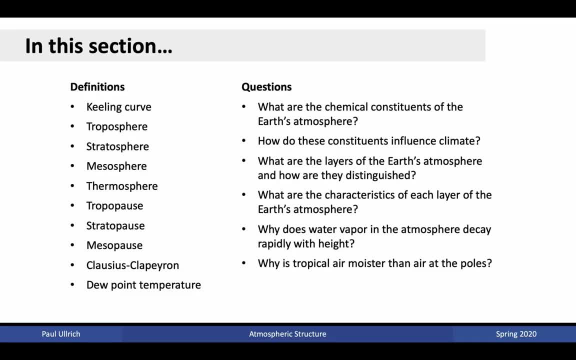 mesosphere and thermosphere, the tropopause, stratopause and mesopause, and the Clausius-Clapeyron relationship and dewpoint temperature. The questions that will be addressed in this section include: what are the key chemical constituents of the Earth's atmosphere and how do these chemical 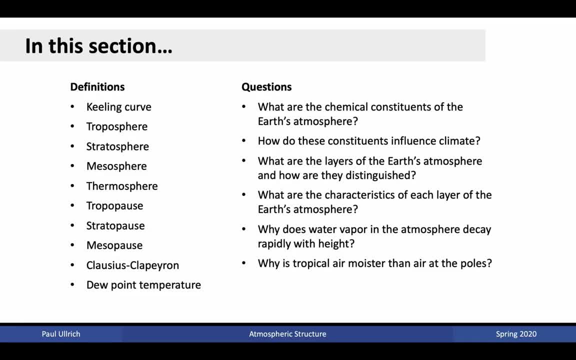 constituents influence the climate system, particularly through energy balance. We're going to discuss the various layers of the Earth's atmosphere and how they're distinguished from one another, as well as the characteristics of each of those layers. Then we're going to talk about the role that water vapor plays in the Earth's atmosphere, in particular, focusing on 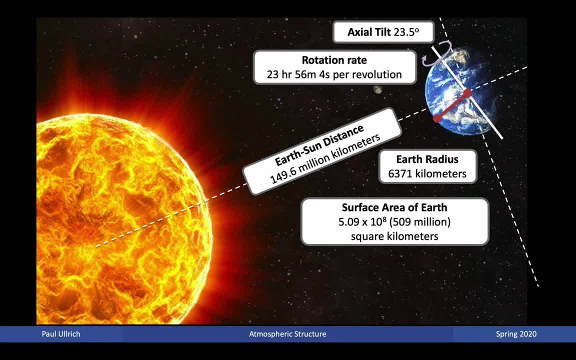 the meridional and vertical structure of water vapor. All right, let's take a very zoomed out view of the whole system, Starting from basics. we know that the Earth is tilted, which enables seasons. We know that it rotates approximately once every 24 hours. We know that the Earth's sun distance 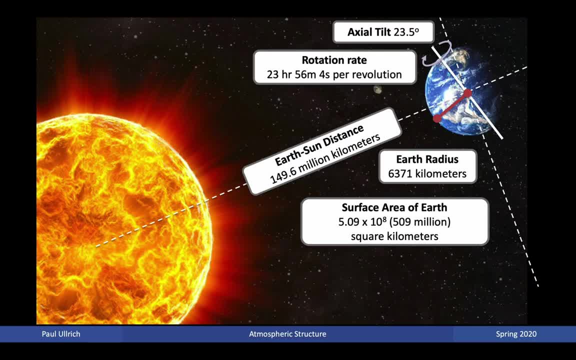 is about 150 million kilometers, and the Earth's radius is about 6,371 kilometers. This allows us to, of course, compute the overall surface area of the Earth. Now, this is just worth keeping in mind as we assess how thick the atmosphere is relative to the Earth itself. 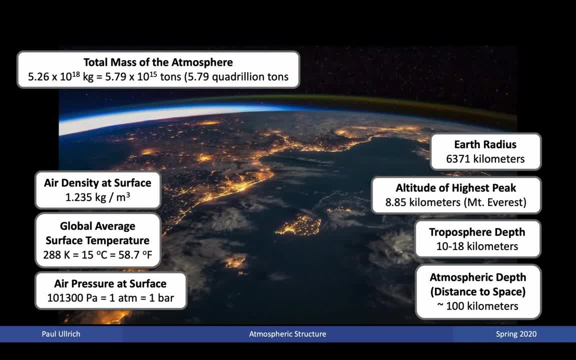 We then zoom in on the Earth. We, of course, can calculate the total mass of the atmosphere, which turns out to be about 5.26 times 10 to the 18 kilograms, or about 5.79 times 10 to the 15 tons. 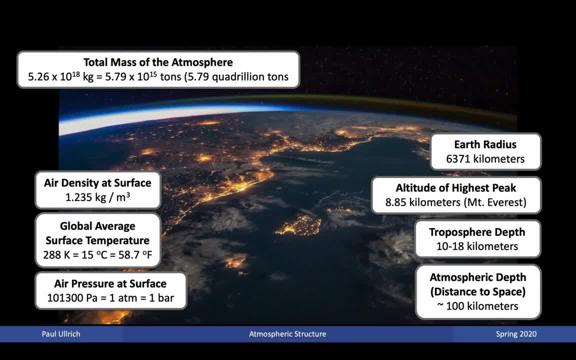 or approximately 5.79 quadrillion tons. The air density at the surface is about 1.235 kilograms per meter cubed, with a global average surface temperature of about 288 degrees Kelvin. Air pressure at the surface, then, is about 101,300. 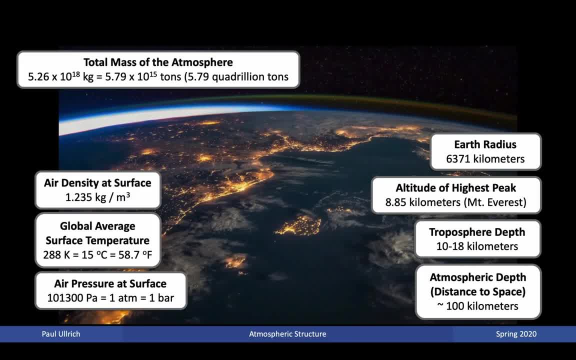 pascals, or about 1013 hectopascals. This is also written as either one atmosphere or one bar. The Earth's radius, as mentioned previously, is 6,371 kilometers and the height of the highest peak on the Earth is about 8.85 kilometers. Given this, actually one. 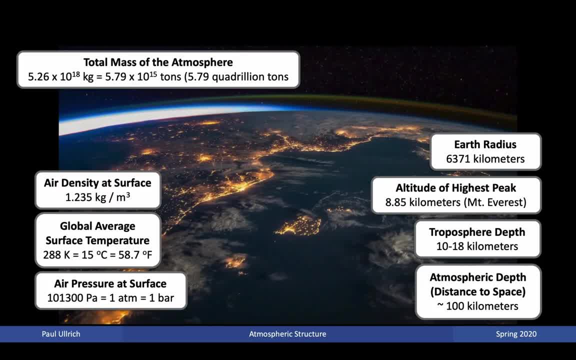 can calculate the overall smoothness of the Earth, and what we find actually is that the Earth is more smooth than even a pool ball, that is, a billiards ball or one that one would typically play with, Which one would typically perceive as being pretty smooth, But the Earth itself is actually. 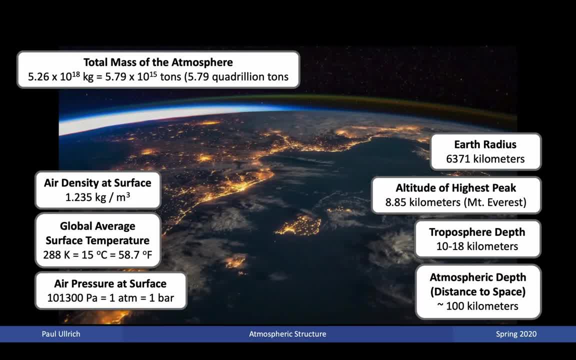 even smoother than that, regardless of the rough topographic variations over its whole surface, However, the atmosphere itself is also a very thin layer. The troposphere, where most of the Earth's weather occurs, actually extends up, at its highest peak, to about 18 kilometers altitude. So comparing that to the radius of the Earth, we see that. 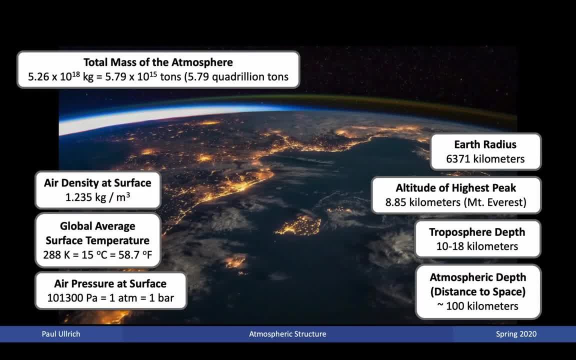 the atmosphere is really just a very, very thin shell. In fact, if one was to extend the atmosphere all the way to what is considered internationally be the distance to space, about 100 kilometers altitude, one again finds that, basically, the atmospheric depth is a small fraction of the total Earth radius. 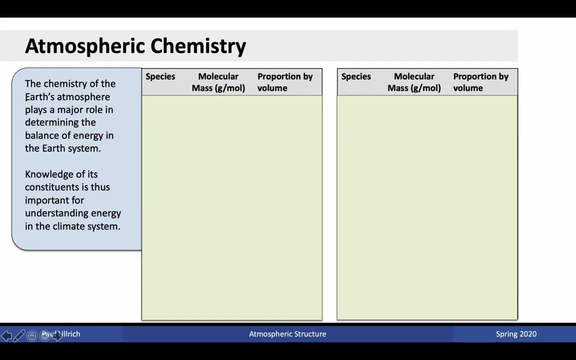 Okay, let's talk about the chemistry of the Earth's atmosphere. As we know, the chemistry plays a very important role in determining the overall balance of energy in the Earth's system. This comes in because different chemical species react differently to different wavelengths of photons. Thus, it is important to understand the constituents of this system in order to 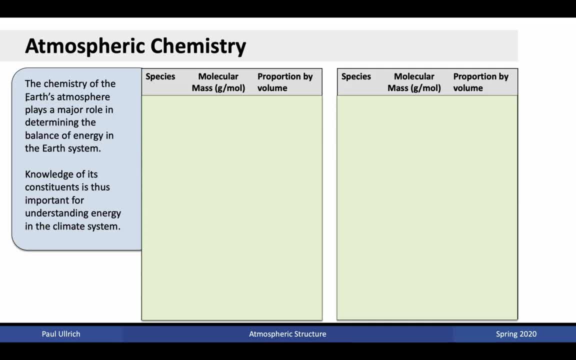 understand overall energy balance. Alright, let's start from the top. As we go through these, you can also quiz yourself on these chemical constituents and compare it against your past knowledge of the composition of the atmosphere. Alright, starting from the top again. the two major constituents of the atmosphere are: 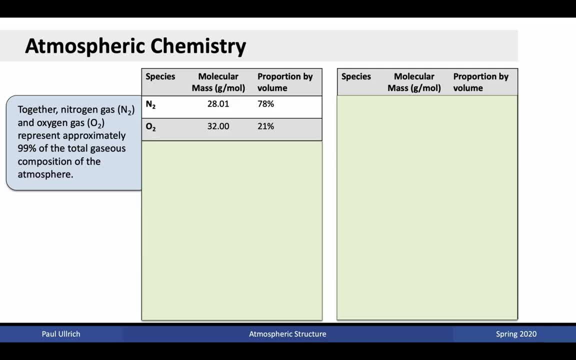 nitrogen gas N2, and oxygen gas O2.. Nitrogen composes approximately 78% of the atmosphere by volume and oxygen gas about 21% by volume. However, nitrogen gas, although it is by far the vast majority of the total gas within the atmosphere, plays very little role in 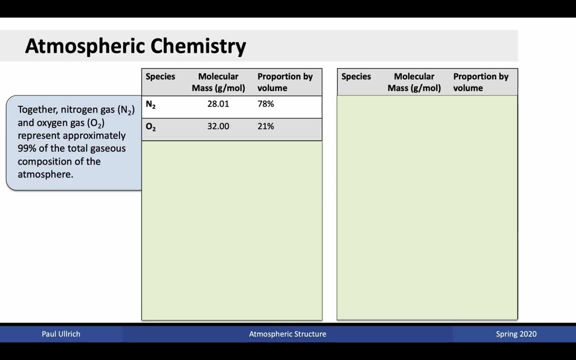 the overall energy balance of the system. Oxygen gas does play some role in the sense that it prevents the highest energy photons from reaching the Earth's surface. This is because oxygen gas is able to absorb incoming high energy photons and disassociate through a process known as the Chapman cycle. This also gives rise to ozone gas and in 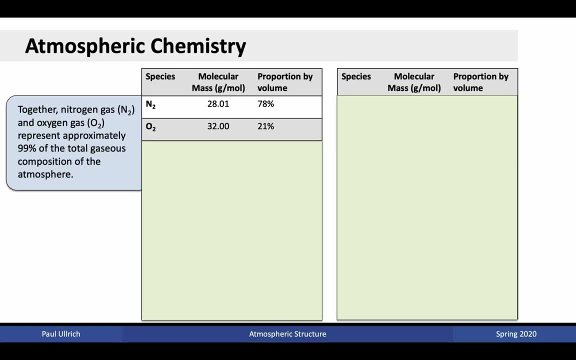 particular forms the ozone layer in the stratosphere. These two species together, then, represent 99% of the total gaseous composition of the atmosphere. The next gas that appears is argon. Argon composes about 0.93% of the atmosphere by. 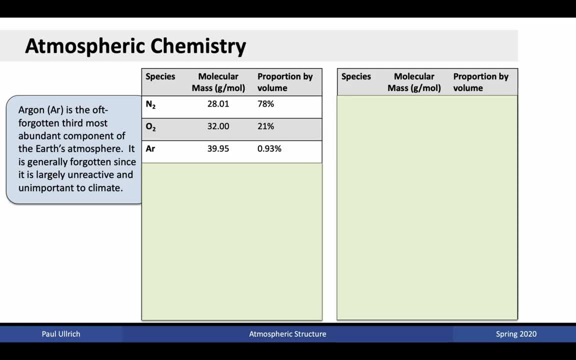 volume, although it is often forgotten because, again, it plays very little role in energy balance of the system and is otherwise an inert gas, so it doesn't involve itself substantially in chemistry either. The next most prominent gas is water vapor, although that's highly dependent on where. 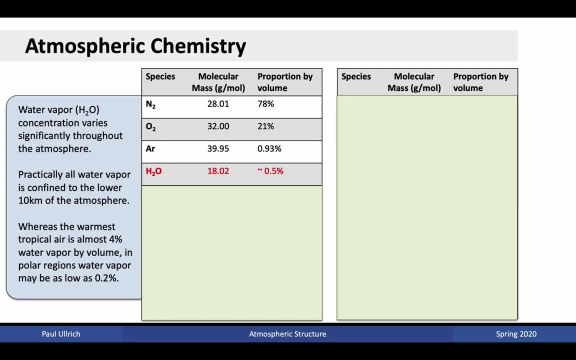 you are and where you are investigating in the Earth's atmosphere. Typically warmer regions also have more water vapor. that's because, as we will see later, the warmer the air is, the more water vapor there is. That means you can see very clearly where 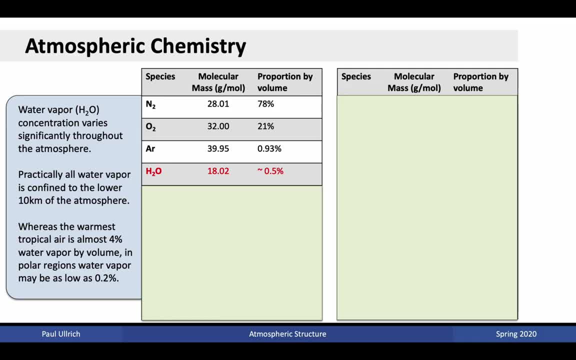 we are just now, vapor than that air can hold. Practically all of the water vapor is confined to the lower 10 kilometers of the atmosphere. This is also related to the fact that this is the warmest region of the Earth's atmosphere. 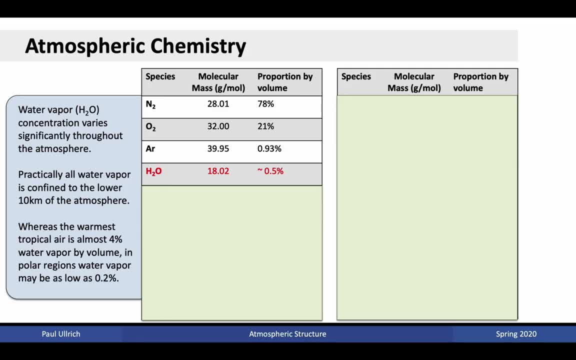 As well. it's next to the source of water which comes from the Earth's oceans. So evaporation from the oceans necessarily enters through the bottom of the troposphere And it's very difficult for that water vapor to be carried up to substantial altitude. 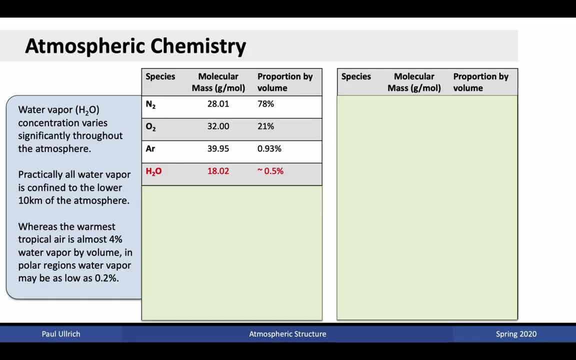 because temperatures drop off substantially with height. Whereas the warmest tropical air is about 4% water vapor by volume, in the polar regions water vapor may be as low as 0.2%. Again, these numbers refer primarily to water vapor found at the surface. 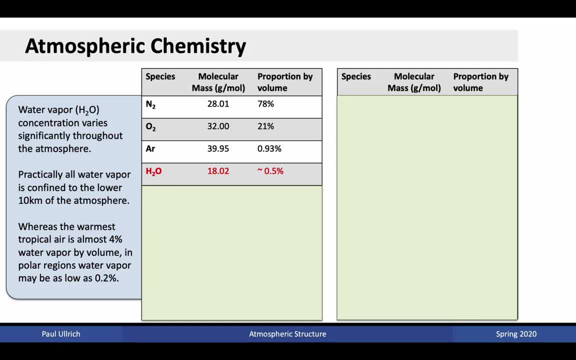 As you go higher and higher up in the atmosphere, the atmosphere quickly becomes very dry and water vapor drops to a mere trace gas. The next most abundant gas in the atmosphere is carbon dioxide, making up approximately 410 parts per million at present. 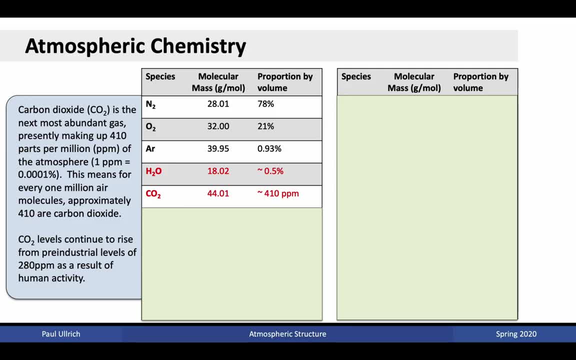 Note: one part per million is equal to 0.0001%. The abundance of carbon dioxide has varied substantially over the past century because of human activities. If we were to go back to pre-industrial times, one would instead find a carbon dioxide abundance. 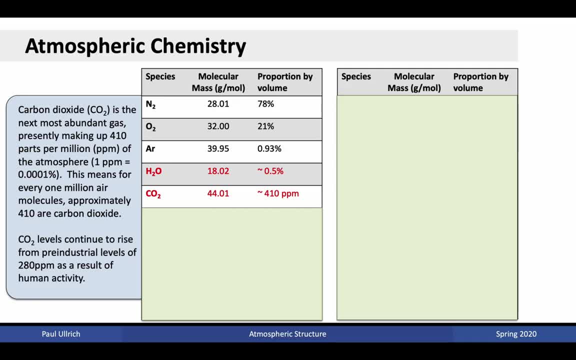 of about 280 parts per million, So that rise of about 130 parts per million can primarily be attributed to human activities. If we continue emitting carbon dioxide at the current rate, it is not infeasible to imagine carbon dioxide rising to nearly 1,000 parts per million. 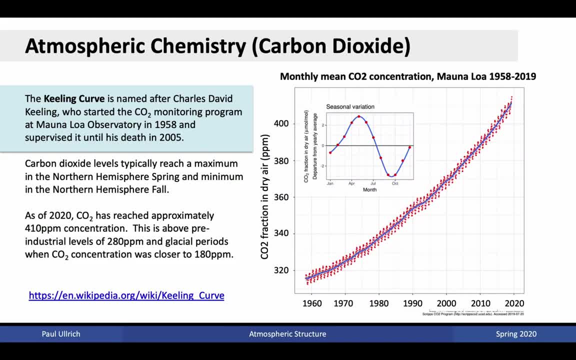 by the end of the century. Atmospheric carbon dioxide concentrations are usually depicted via the Keeling curve. This gives a historical time series of carbon dioxide as measured at the Mauna Loa Observatory. The Keeling curve is named after Charles David Keeling, who 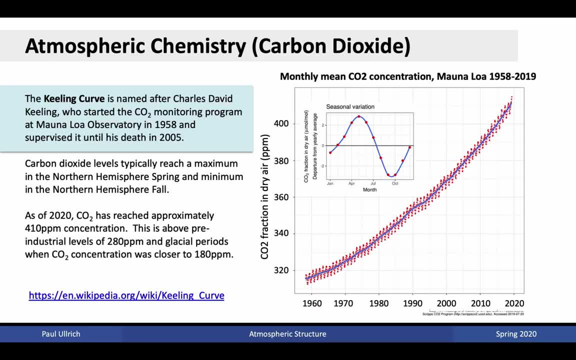 started the carbon dioxide monitoring program at the Mauna Loa Observatory in 1950.. The Keeling curve is named after Charles David Keeling, who started the carbon dioxide monitoring program at the Mauna Loa Observatory in 1950.. The Keeling curve is named after Charles David Keeling, who started the carbon dioxide monitoring program at the Mauna Loa Observatory in 1950.. 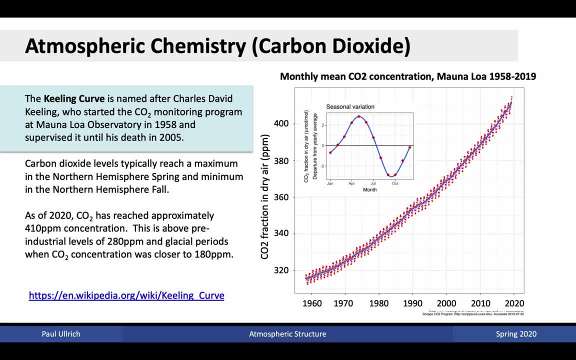 and supervised it until his death in 2005.. This system continues to monitor carbon dioxide levels through today. Carbon dioxide varies substantially throughout the season because of vegetation growth on the Earth's surface. Because the Northern Hemisphere has more land area, it also is associated with more carbon dioxide uptake. 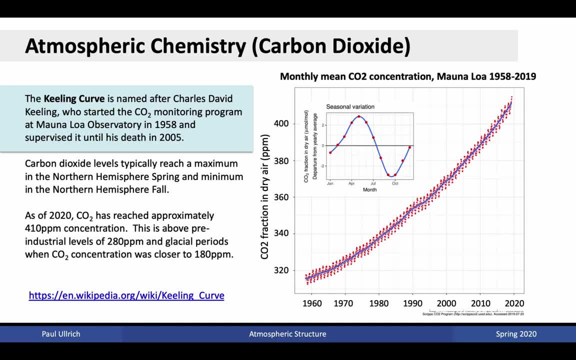 Consequently, carbon dioxide levels typically reach a maximum in the Northern Hemisphere spring. then, as vegetation grows throughout the season and uptakes carbon dioxide, we see a drop in overall carbon dioxide levels. Minimum levels are then reached in the Northern Hemisphere, fall As vegetation in the Northern Hemisphere dies out. 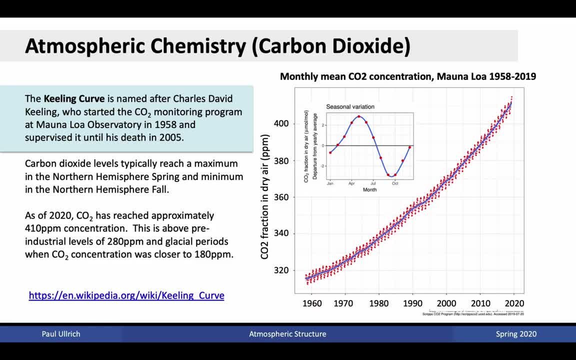 we see a return of carbon dioxide to the atmosphere. As of 2020,, carbon dioxide has reached approximately 410 parts per million concentration, so these slides will have to be updated in future years as carbon dioxide levels continue to grow. Going back to pre-industrial times, we saw numbers at about 280 parts per 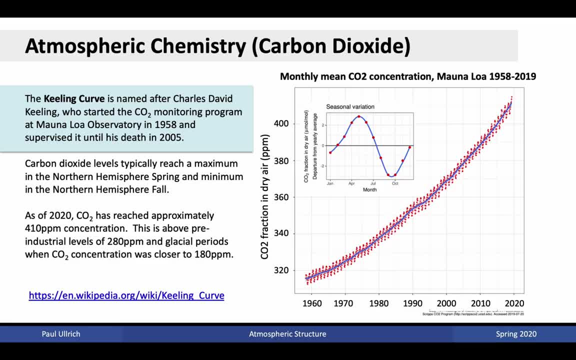 million. When the original observations were made in 1958 at Mauna Loa Observatory, numbers were approximately 315 parts per million. Going back even farther into the past, one finds that during the glacial periods in the Earth's history, carbon dioxide concentrations were much closer to 180 parts per million. 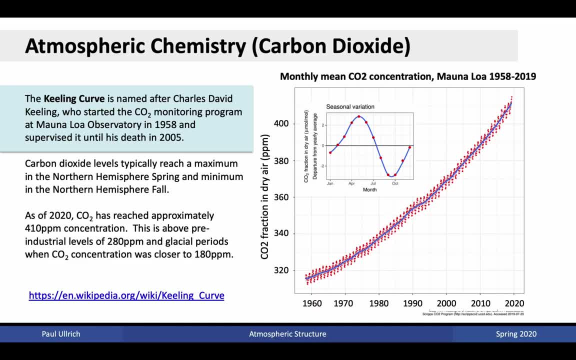 It turns out that carbon dioxide and surface temperatures are closely correlated with one another. hence why it is worrying that we see such a dramatic increase in carbon dioxide over the past century. Alright, returning to our examination of the chemistry of the Earth's atmosphere. 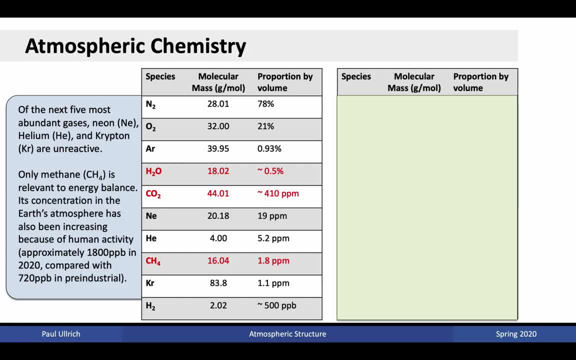 we're now in the bottom phase of this first column. What we see next is Neon, Helium, Methane, Krypton and Hydrogen. Of these, three of them are noble gases and hence are largely non-reactive and not really of particular interest for energy balance in the Earth's system. 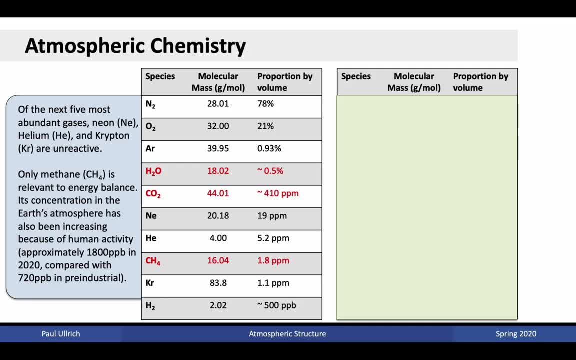 Only methane is really important to energy balance as a powerful greenhouse gas. The Earth's atmosphere has also seen a dramatic increase in methane levels because of human activity. As of 2020, it's approximately 1,800 parts per billion or 1.8 parts per million. 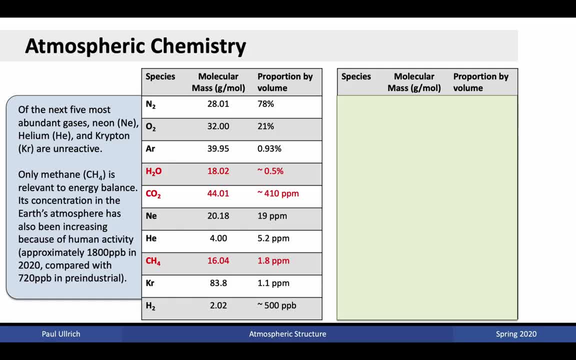 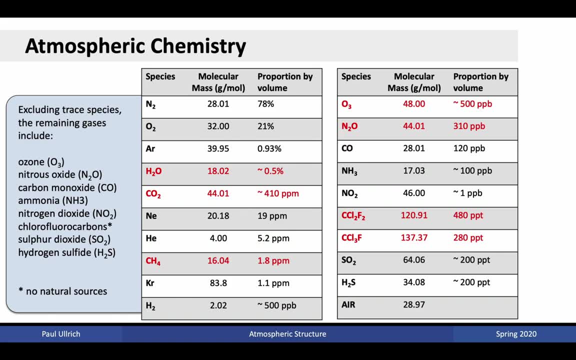 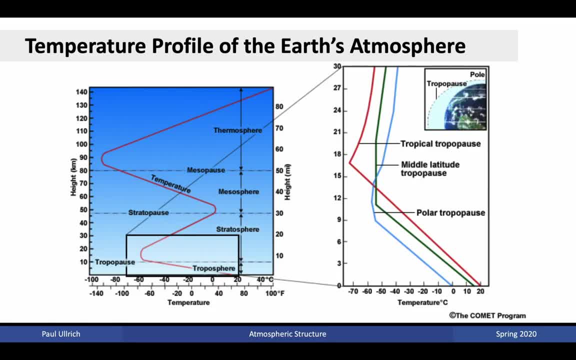 In the mid-latitudes we see warmer surface temperatures, but a tropopause temperature that is approximately the same as that of the polar tropopause. In the tropical regions we see the warmest surface temperatures, but because of convective uplift that pushes up the tropopause in this region. 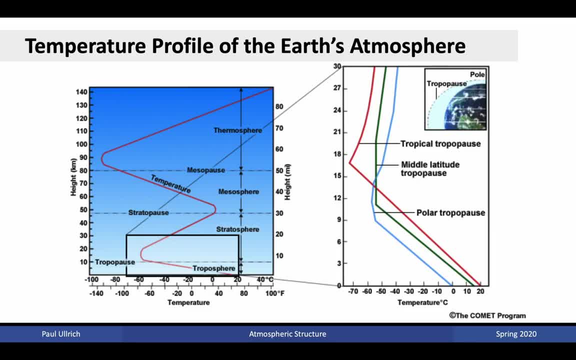 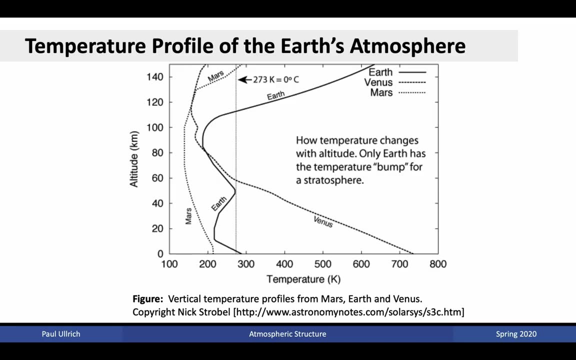 we also see that this trend of decreasing temperatures tends to go farther up in the atmosphere. Consequently, the tropical atmosphere tends to reach the coolest temperatures overall near the tropical tropopause. Comparing Earth to some of its companion planets, specifically Mars and Venus, we find that the Earth is fairly unique in this distribution of vertical temperatures. 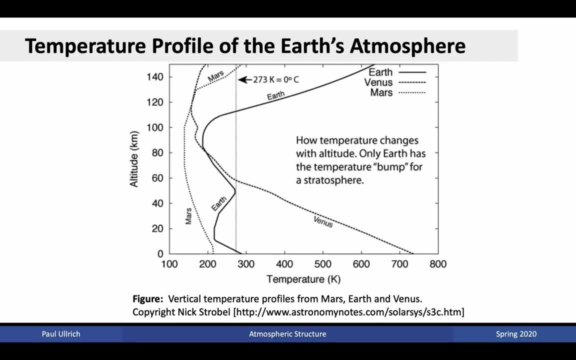 Earth is the only planet that sees a bump in the stratosphere. Mars, on the other hand, basically sees a decrease in temperatures through its Martian troposphere and an increase in the temperature of the stratosphere. The same is pretty much true for Venus. 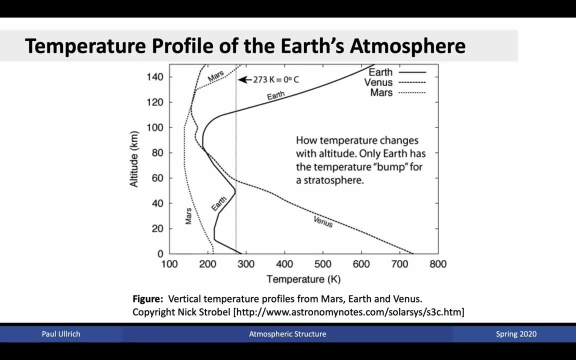 Although it has much warmer surface temperatures. effectively it has a decrease in temperatures with altitude until you reach the top of its troposphere, and then an increase as you get to higher altitudes. This presence of the bump in the Earth's vertical temperature profile can be attributed purely to the chemistry of the Earth's atmosphere, as we'll see shortly. 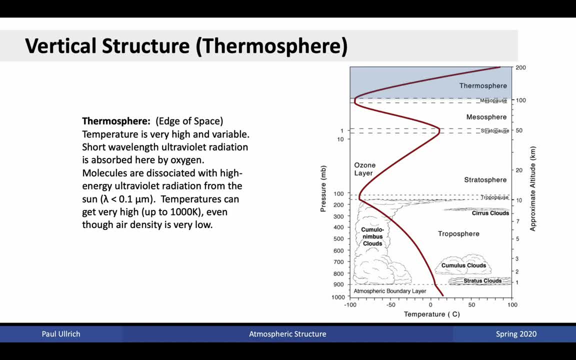 Alright, let's start at the top of the Earth. Let's start at the top of the Earth's atmosphere and work our way down to the surface. The thermosphere is considered to be the edge of space. Temperatures here are very high and very variable. 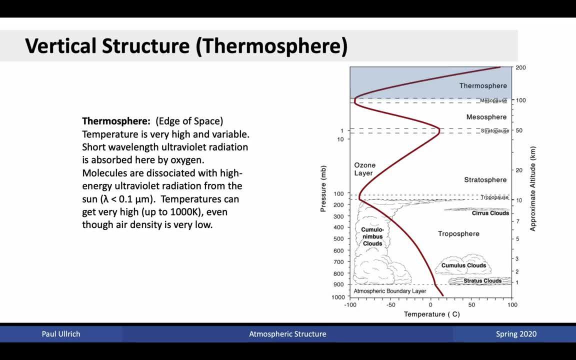 That is, they vary heavily depending on whether you're on the dark side of the planet or the light side of the planet. It is also a region which is effectively exposed to solar radiation in its highest concentrations, including some of those highly energetic photons that are notorious for being cancer-causing agents. 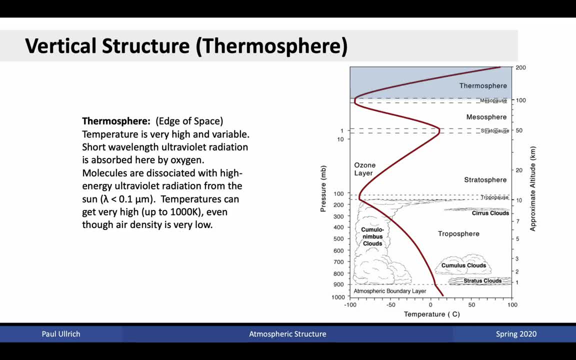 This high-energy ultraviolet radiation is a region that is very high in temperature, and it's very high in temperature Also, it is very low in atmospheric order In general호I. unwanted radiation also tends to disassociate molecules, leading to ionization of gases at this altitude. 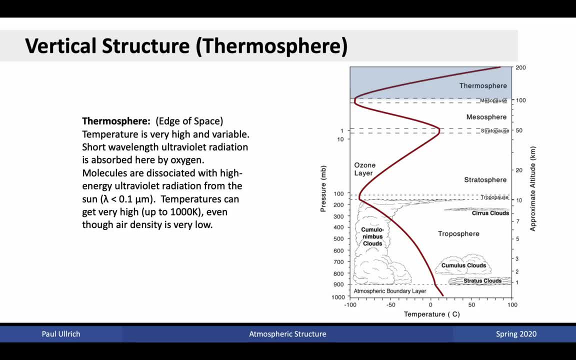 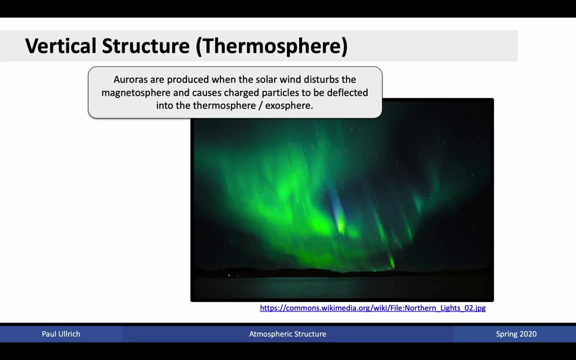 Although temperatures can get very high, particularly through the top of the thermosphere, the air density is very low, so you wouldn't necessarily feel it In the thermosphere. the solar wind is able to disturb gasses at higher altitude and deflect particles into the thermosphere and exosphere. 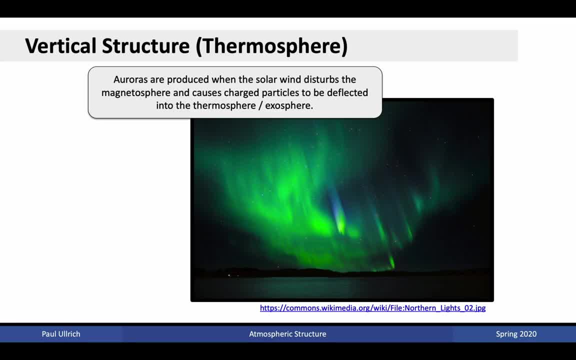 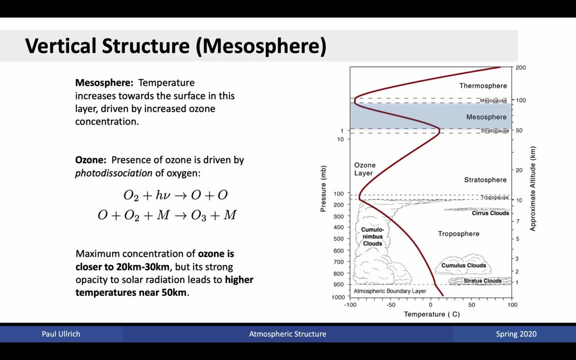 This process then acts like a constant thermal reaction taking place in the atmosphere. This process then acts like a constant thermal reaction taking place in the atmosphere, gives rise to what are known as auroras or the northern lights. Below the thermosphere is the mesosphere. Temperatures tend to increase towards. 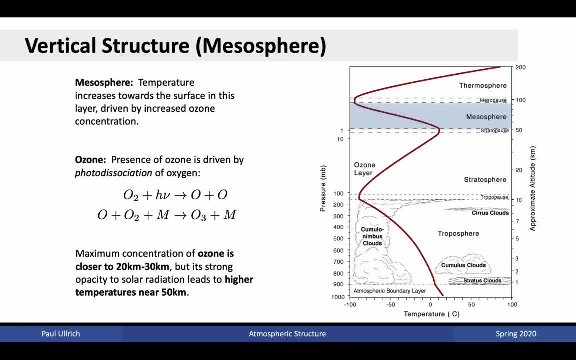 the surface in this region, as we observe higher concentrations of oxygen gas and consequently higher concentrations of ozone. As highly energetic particles photons from the Sun enter the Earth's atmosphere, they're able to disassociate oxygen gas in order to form individual oxygen atoms. These oxygen atoms can then 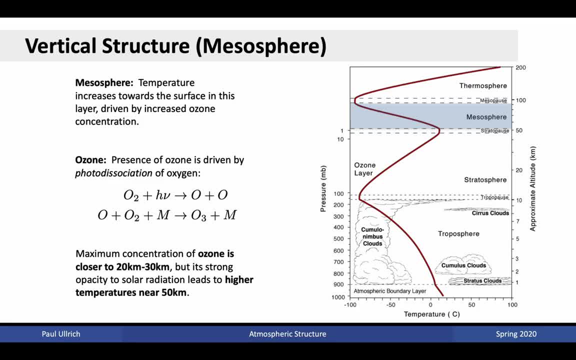 combine with oxygen gas in order to produce ozone. Through this region we see much of these highly energetic photons that are able to disassociate the oxygen gas, decrease in density as we go farther down. as they collide with oxygen gas within the atmosphere, The maximum concentration of ozone is closer to. 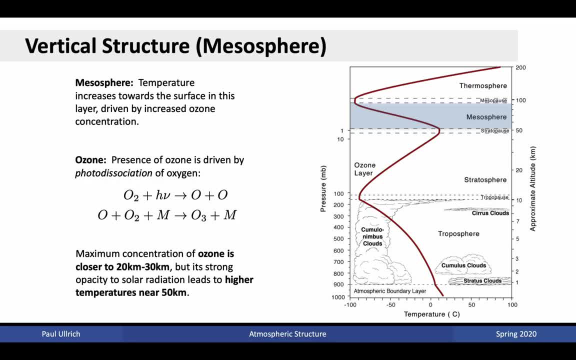 about 20 or 30 kilometers, nestled between the atmosphere and the atmosphere and directly within the stratosphere. but its strong opacity to solar radiation actually leads to the highest temperatures occurring at about 50 kilometers altitude. So the thermal maximum of the atmosphere is not. 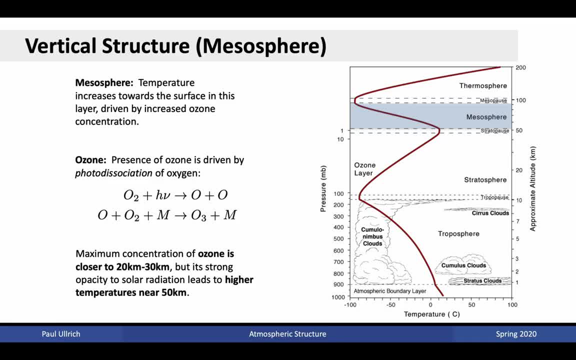 co-located with the maximum density of ozone. Keep in mind, ozone is produced because of a combination of two factors. One is purely the density of oxygen gas, which increases as you go closer towards the surface, and the density of highly energetic solar photons, which increase the density of oxygen gas. The density of oxygen gas is 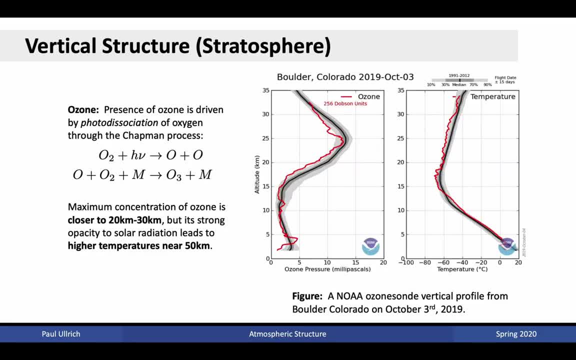 reduced as you go closer towards the surface. As one enters into the stratosphere, we see that ozone becomes essential in determining this underlying temperature profile. As we enter the region of highest concentration of ozone, we actually find that temperatures are decreasing as we move our way towards the surface. As mentioned previously, the maximum 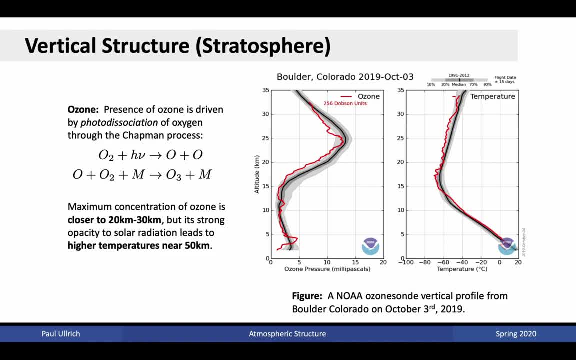 concentration of ozone appears at approximately 20 to 30 kilometers altitude. Shown on the right here are ozone-assoned vertical profiles obtained from Boulder, Colorado. Although the ozone tends to be highly variable, we see this fairly consistent profile around the Earth's surface. 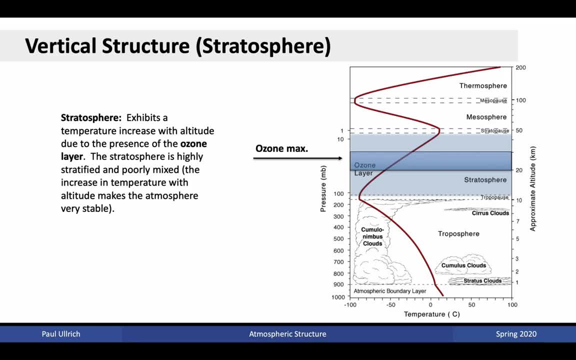 Alright, let's talk about the stratosphere. Through the stratosphere, temperatures decrease as one moves closer towards the surface. The stratosphere tends to be highly stratified and poorly mixed Because of the particular temperature profile. there tends to be very little rise in temperature. 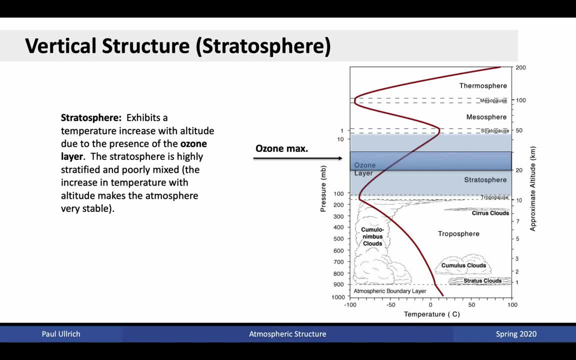 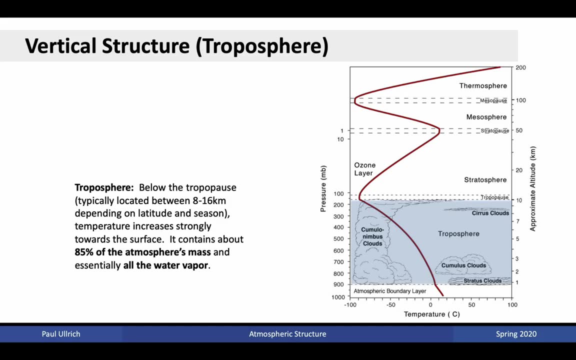 The stratosphere has a lot of rising or sinking motion occurring within this layer, and so it's very difficult for air to move up and down. Consequently, air within the stratosphere can persist there for a very long time. The ozone layer is located within the stratosphere as well, as mentioned previously As one. 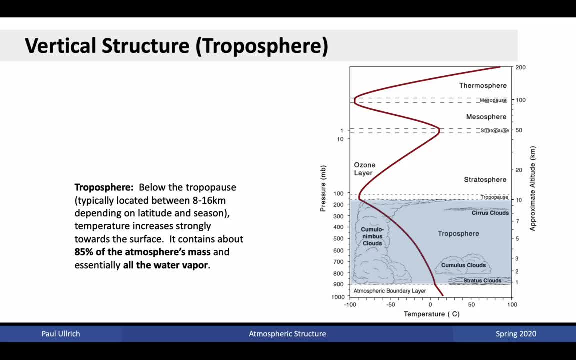 moves below the stratosphere, we encounter the tropopause and then enter into the troposphere. The troposphere occurs between approximately 8 and 16 kilometers altitude. The stratosphere on the right is very approximate, as the tropopause varies substantially depending on your particular latitude In the tropics. the 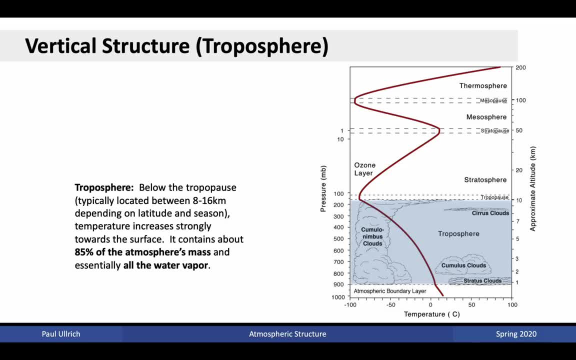 tropopause can reach altitudes of nearly 20 kilometers, whereas in polar regions the tropopause occurs at approximately 8 kilometers. Again, this is just simply a region where temperatures are effectively constant with altitude. The troposphere contains about 85 percent of the atmosphere's mass, accounting to the 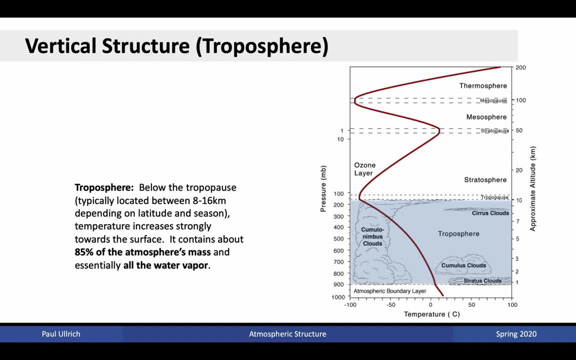 fact that as one moves closer towards the surface, you simply get a higher density. This is because gravity is effectively pulling the atmosphere towards the surface. It is also it contains essentially all of the Earth's water vapor. That is again because you have evaporation from the 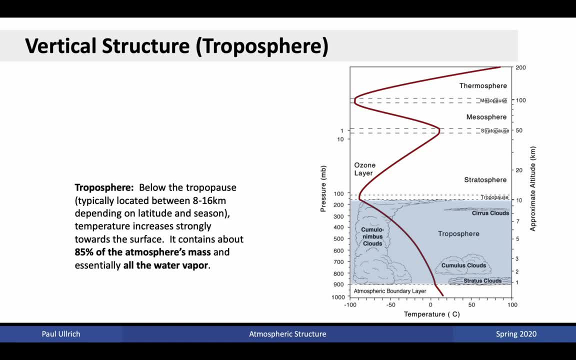 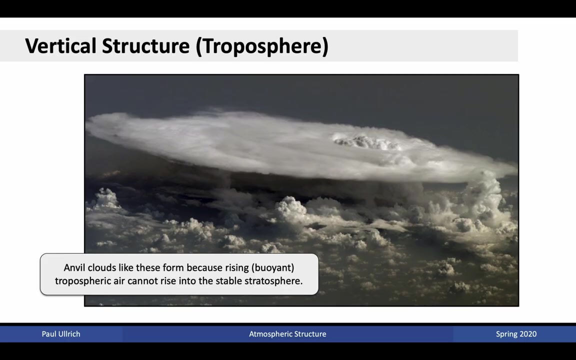 surface, and hence water vapor entering in through the bottom of the troposphere. It becomes very difficult, through the higher altitudes of the troposphere, for water to be maintained in vapor form, as cooler temperatures tend to give rise to condensation of that vapor And hence precipitation. The troposphere is home to our large weather events In. 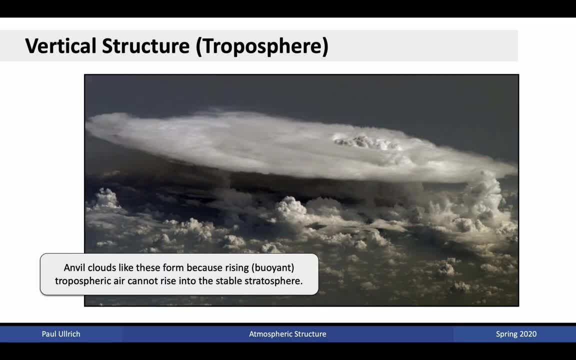 particular, we can see things like a cumulonimbus cloud here, an anvil cloud that forms because of rising motion. Basically, you start with a warm, moist bubble near the Earth's surface that initiates convection. This rising motion then carries with it the moisture from the near Earth's surface and as that, 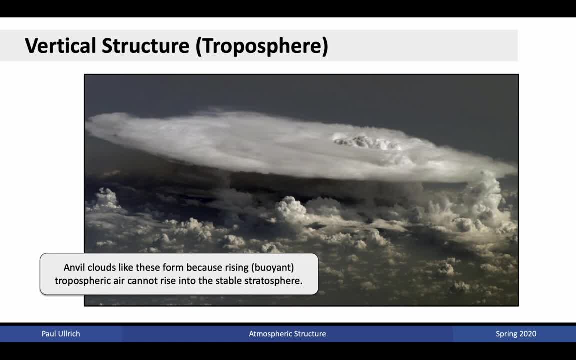 reaches its condensation level, we get cloud droplets that form. These cloud droplets consist of liquid water. As the parcel rises, it eventually can hit the tropopause. At the tropopause it is unable to rise any farther, as we'll discuss in our 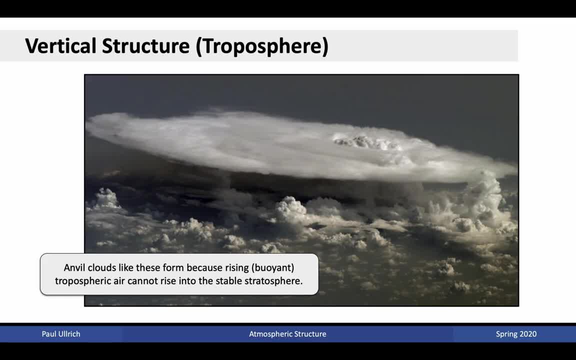 lecture on convection. Consequently, you get a spreading out of water vapor away from this point. The flat top of the anvil clouds hence is typically the bottom of the anvil, the top of the anvil, the top of the anvil and the top of the anvil. 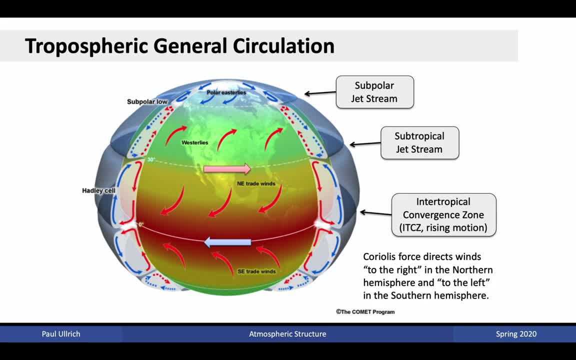 The top of the anvil is the most common part of the anvil. The top of the anvil is the most common part of the anvil Throughout the troposphere. we also have the tropospheric general circulation, or what is more commonly just referred to as the general circulation of the planet. 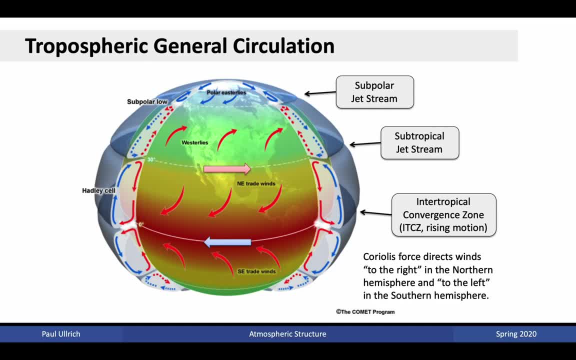 It turns out that we have, in each hemisphere of the planet, three major cells which circulate air horizontally. This enables the exchange of heat between the tropical regions, where we have most of our insulation, and the polar regions, which tend to be cooler, receiving less insulation. Weather patterns, then, are associated with the redistribution of heat. 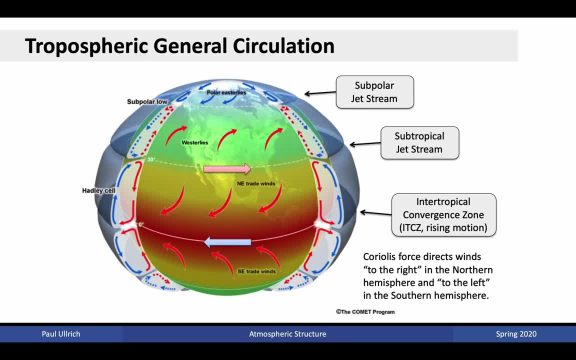 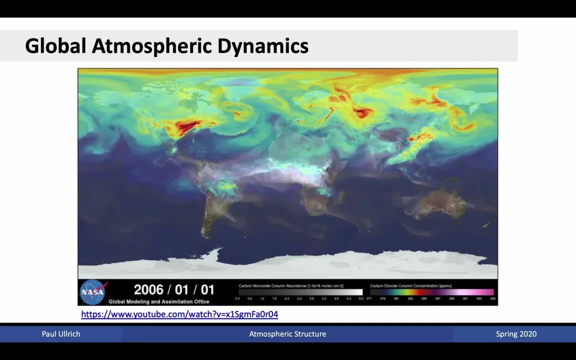 from these tropical regions to polar regions. The general circulation arises naturally because of the presence of Coriolis force and this temperature gradient across the surface. We'll go into more detail about the general circulation of the planet in lecture 5.. Global atmospheric dynamics are largely present within the troposphere, and it's the most 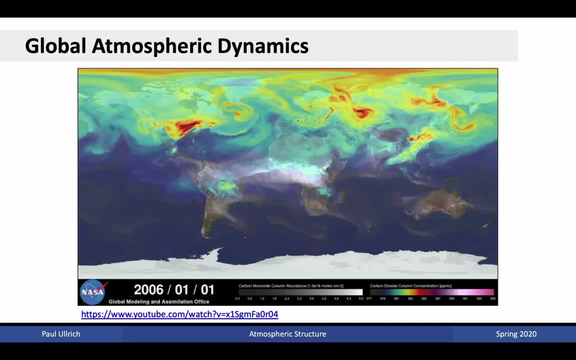 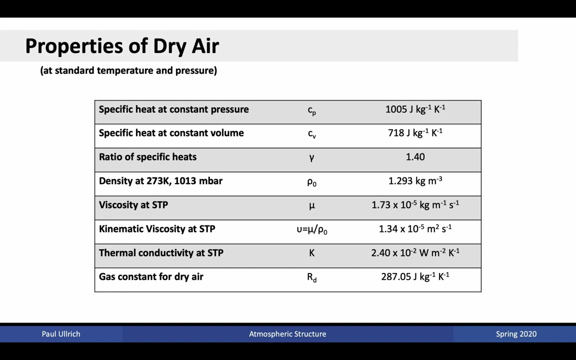 important for us, as we live in the troposphere. Hence, an understanding of weather patterns within this region and how air movement gives rise to these weather patterns is important for understanding the weather that will affect us, as well as understanding the underlying climate system. All right, let's talk about water vapor in the atmosphere. Here are some properties that: 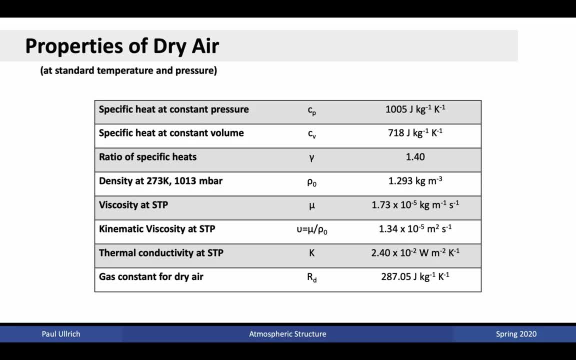 will be relevant for potentially future assignments. What is worth noting about dry air is its specific heat capacity, which determines how much energy is needed to increase the temperature of dry air, and we'll see how this contrasts with water vapor. Other quantities that are relevant for understanding the dynamics include the viscosity. 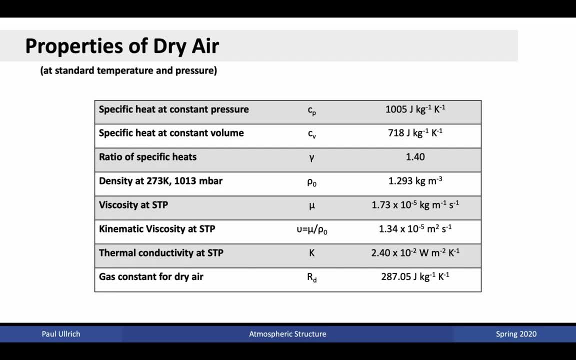 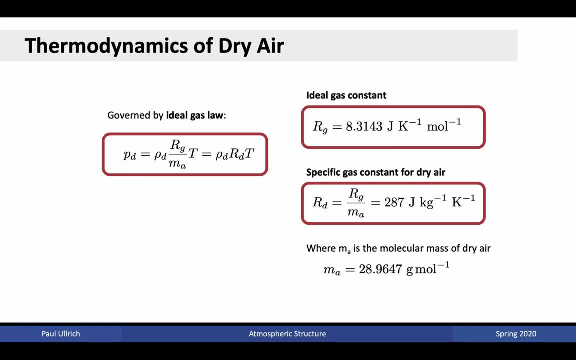 of the air, as well as thermal conductivity and its ideal gas constant. All right, let's review briefly the thermodynamics of dry air. Dry air is governed by the ideal gas law, which allows us to relate the pressure of dry air to its density and temperature. 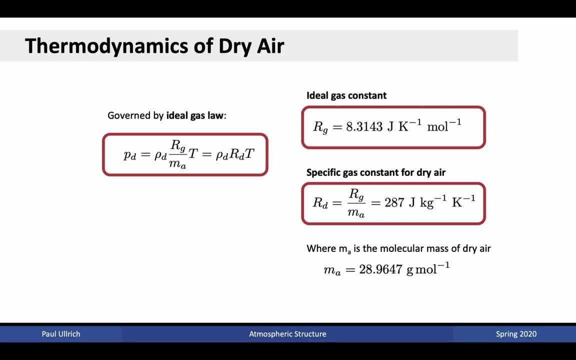 These are proportional via the constant of proportionality, known as the specific gas constant for dry air. This can be obtained by taking the ideal gas constant, which is consistent for all ideal gases, and dividing that by the molecular mass of dry air calculated previously from the chemical composition of the Earth's atmosphere. This gives a value of 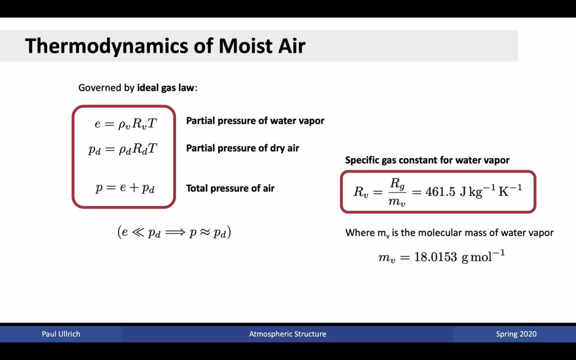 7.27 joules per kilogram per degree kelvin. Moist air is analogously governed by an ideal gas law. Here we are more concerned with the partial pressure of water vapor, that is, the contribution of water vapor pressure to the total pressure of the air. Taking the partial pressure of 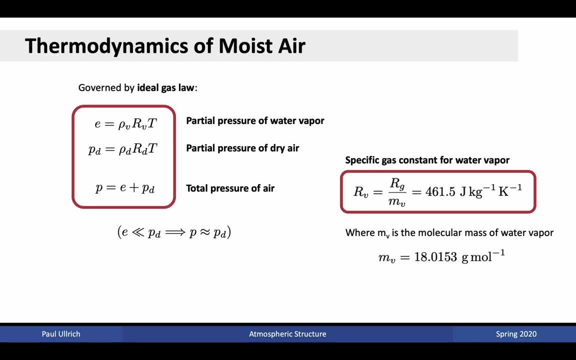 water vapor and adding the partial pressure of dry air gives the total pressure of air. The partial pressure of water vapor is analogously governed by the partial pressure of the air. Usually, if you placed the retainer on a mineral side, the partial pressure of the water would. cover how much air would flow. This also has to do with a partial pressure of the однаiding stores, For example the total pressure plus the amount of the water vapor, hour or air could be a kind of aів and the difference. 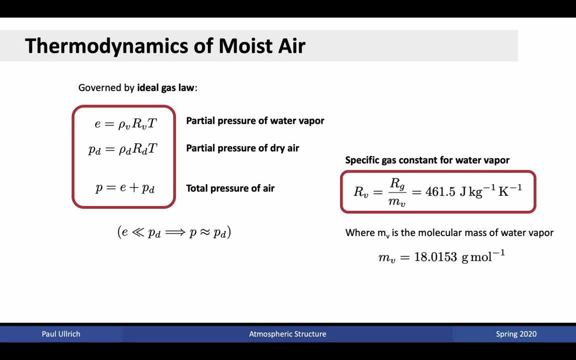 So that how even job is not explained. but at least I hope that this brokenrical definition of crucial respect would be regarded as important, obtained through an ideal gas law relationship associated with water vapor. Here we have the partial pressure of water vapor on the left hand side, typically denoted with letter E. We have the 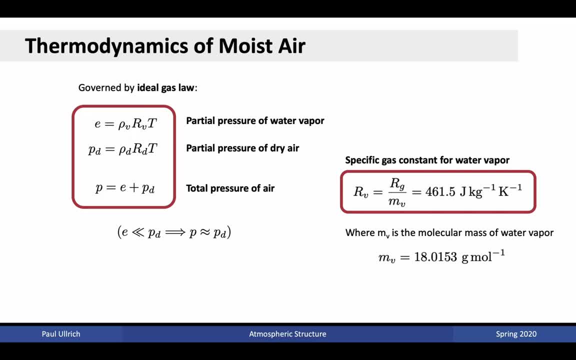 density of water vapor. We have the ideal gas constant or the specific gas constant for water vapor, denoted R, subscript V, and the temperature of the gas. The specific gas constant for water vapor is higher than that of dry air because water vapor is lighter than dry air. Its value, 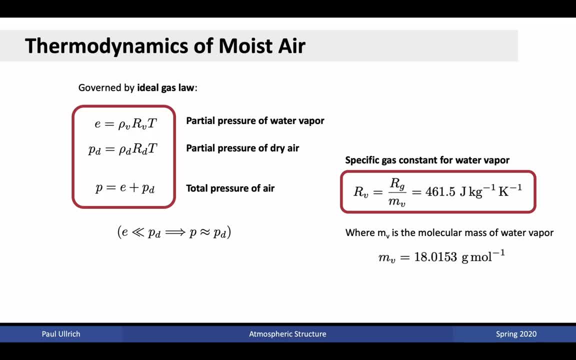 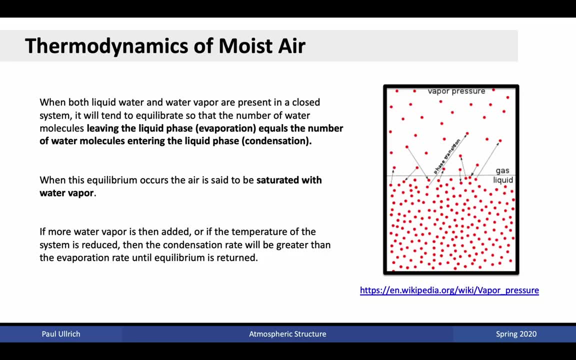 comes out to be approximately 461.5 joules per kilogram kelvin. When you have both liquid and water vapor that are present in a closed system, it tends to equilibrate. This is very important in understanding evaporation and energy balance, as well as understanding condensation within the. 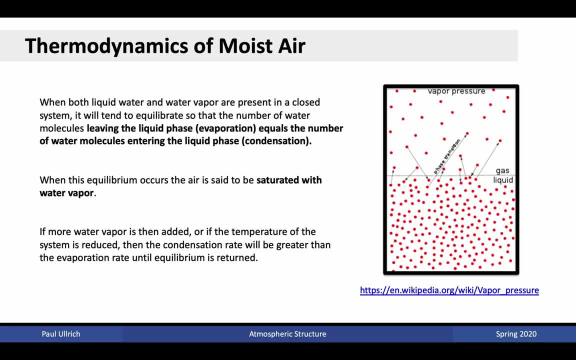 earth's atmosphere. Typically, you have individual molecules of water vapor that can exist in either vapor phase or liquid phase, and at the surface between that gas and liquid, you have molecules that are continuously exiting the liquid phase as well as molecules that are entering the liquid phase. When equilibrium occurs, that refers to the state. 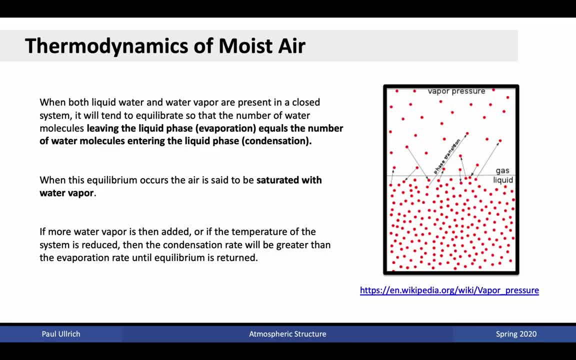 at which molecules are leaving the liquid at the same rate that they are entering the liquid. At this point, it is said that the air is saturated with water vapor. If the air is saturated with water vapor, it is said that the air is saturated with water vapor. 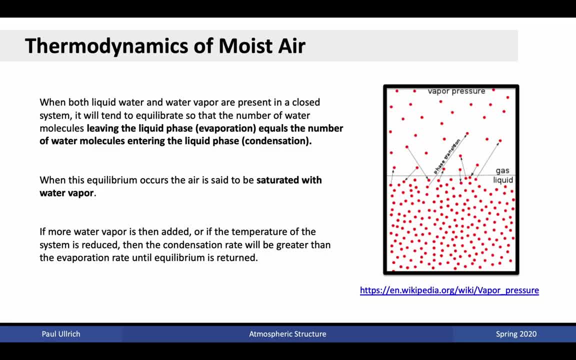 If more water vapor is added in its gaseous form to the gaseous region, you will have an overabundance of gaseous water vapor molecules. Hence you will have more molecules entering the liquid phase than you will have molecules leaving the liquid phase, and it will attempt to re-equilibrate with. 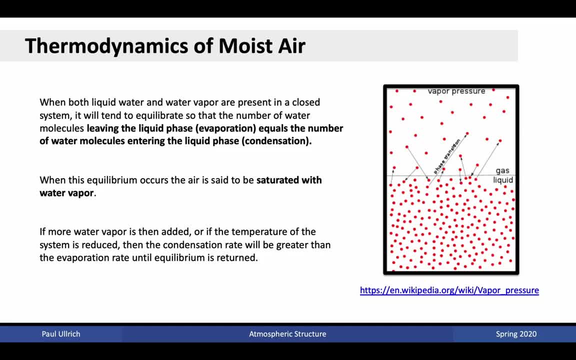 more water in the liquid phase. This will then cause condensation to occur. The amount of water vapor that a gas can hold is determined through is a function of the temperature of the gas, So at lower temperatures, typically, water vapor will tend to condense. That is water. 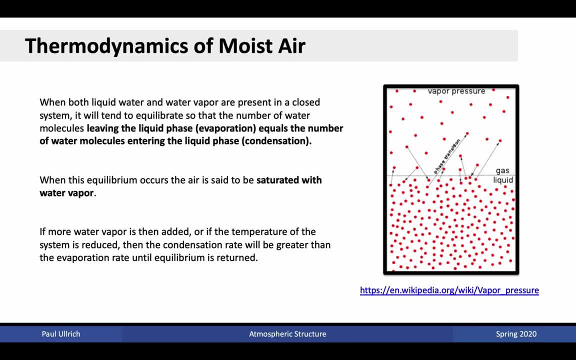 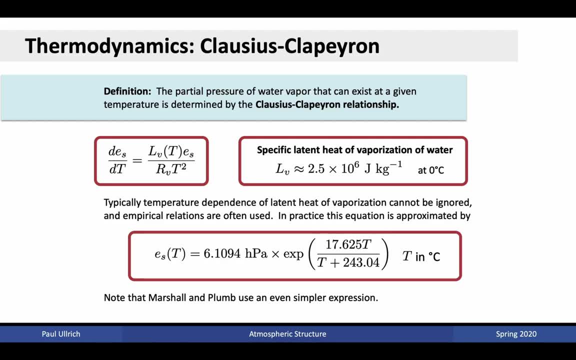 will prefer to exist in the liquid phase over the gas phase, and so you'll have a drop in the water vapor partial pressure within the gas. The amount of water vapor that can actually be held within the gas is determined by what is known as the Clausius-Clapeyron relationship. I'm going to 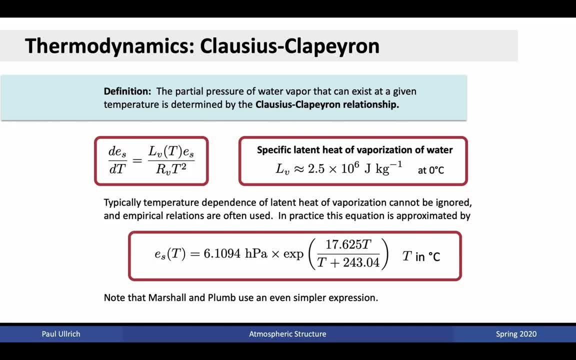 avoid going through the derivation of this particular relationship, because I don't want to go into the relationship, except to say that the water vapor partial pressure at saturation is effectively purely a function of the temperature of air and it can be represented through the differential equation depicted here on the top left. Here Lv denotes the specific latent heat of 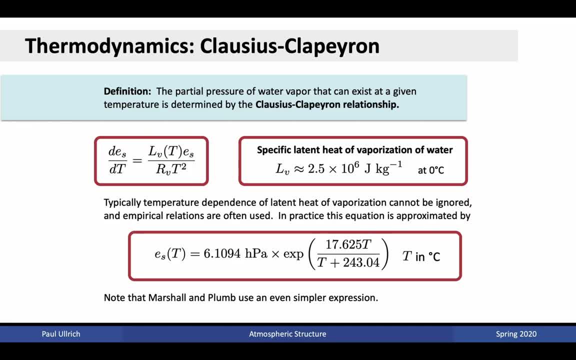 vaporization of water, which effectively refers to how much heat is released when the water vapor evaporates. The equation on the top left here can be solved, but it is worth noting that Lv does have a temperature dependence associated with it, although it's typically approximated by the value shown here. 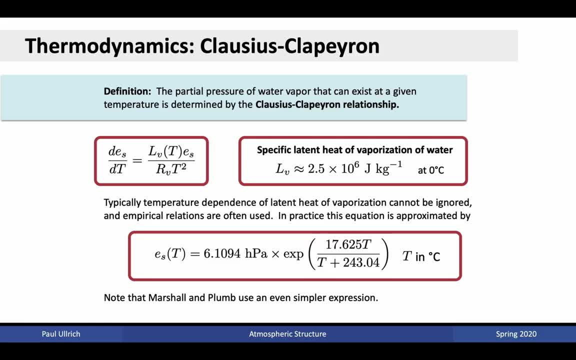 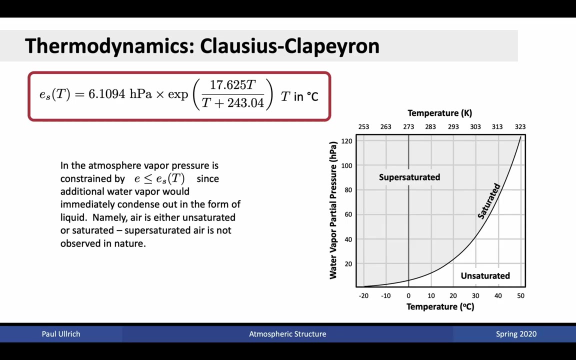 However, one can obtain a more accurate approximation to the saturation vapor pressure through the expression shown below. This is actually a very commonly used approximation for that saturation vapor pressure. If one plots the saturation vapor pressure, one finds that it looks very analogous to an exponentially increasing curve. Water tends to exist in the unsaturated region in the bottom right hand of this diagram. 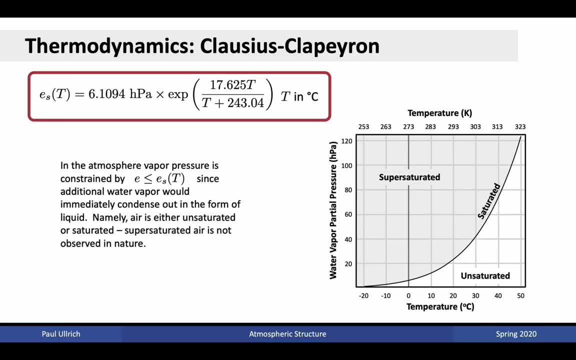 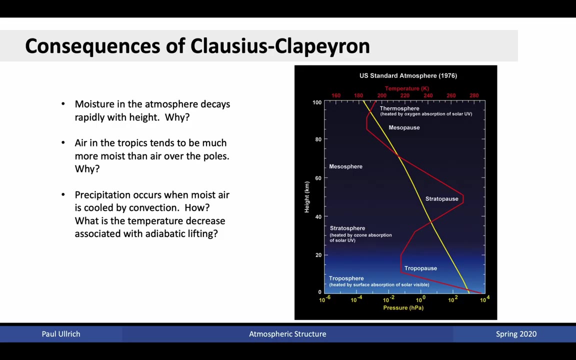 For if the water vapor content enters into the supersaturated regime which is shown here in gray, it will tend to condense. until that water vapor hits the saturated line. Supersaturated air is not typically observed in nature. Alright, so with Clausius-Clapeyron in hand, we can then explain the behavior of water vapor within the atmosphere. 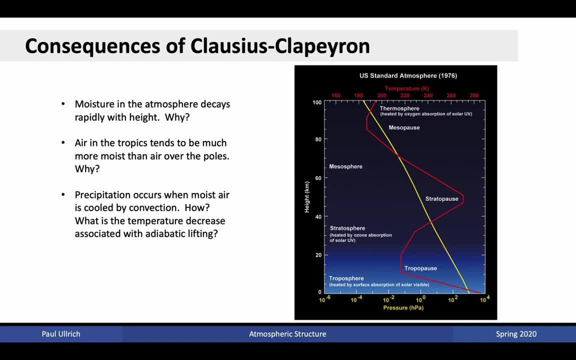 Since we know that the temperature drops roughly linearly through the troposphere, we also then know that the water vapor content must drop as well. In fact, it drops roughly exponentially fast with this drop in temperature. So one then expects that most of the water vapor will be found within the atmosphere. 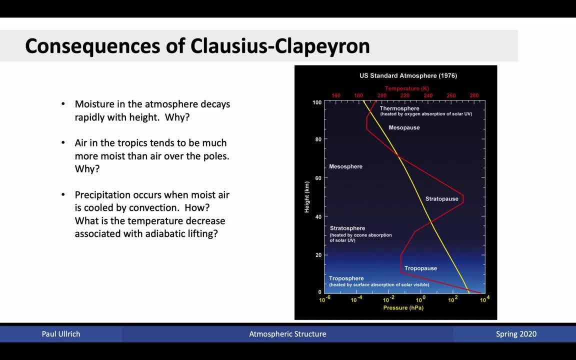 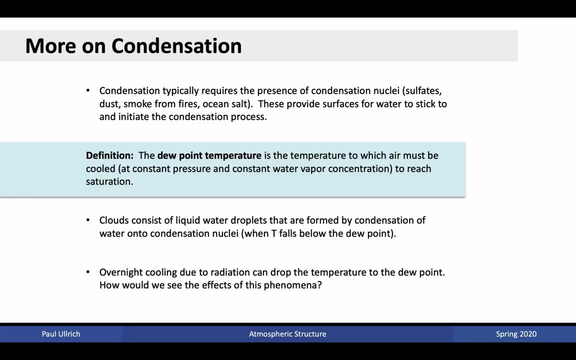 This means that the water vapor will be found near the surface, where temperatures are relatively warm. Analogously, one expects that you will have the highest water vapor concentrations in the tropics, where water vapor saturation pressure tends to be highest. Condensation typically occurs whenever you have condensation nuclei present. 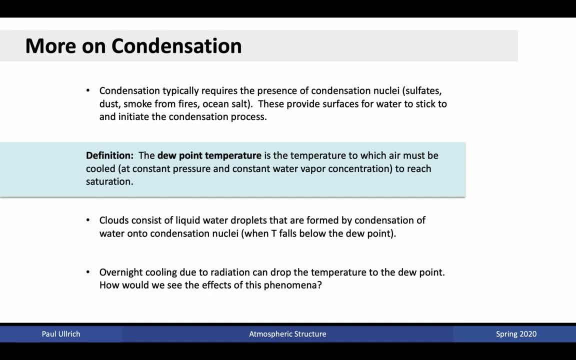 Condensation can occur in a pure water vapor situation, but it tends to be much more difficult, And in those situations you can have water vapor that does exceed 100% relative humidity. However, it tends not to exceed it by very much before condensation does occur. 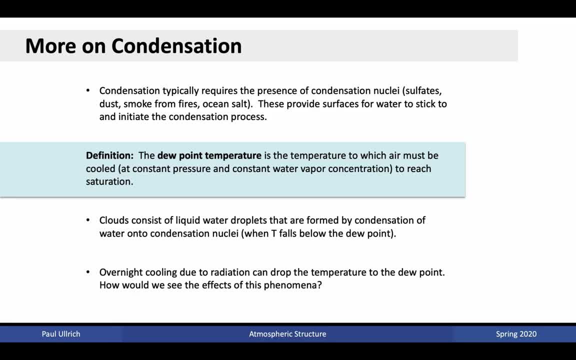 Such a situation again is known as a supersaturated fluid, And in these situations any small perturbation of the system can then trigger condensation. However, condensation in the presence of condensation nuclei often occurs effectively at 100% relative humidity. 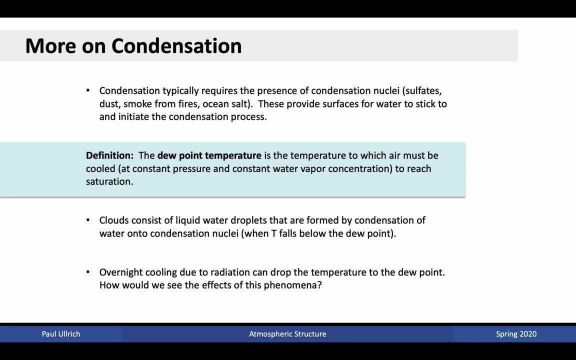 With the condensation nuclei, including sulfates. dust, smoke from fires, ocean salt and other aerosols provide surfaces for the water to stick to and initiate the condensation process. Hence, when one talks about cloud droplets, we typically have a condensation nuclei located at the center of those cloud droplets. 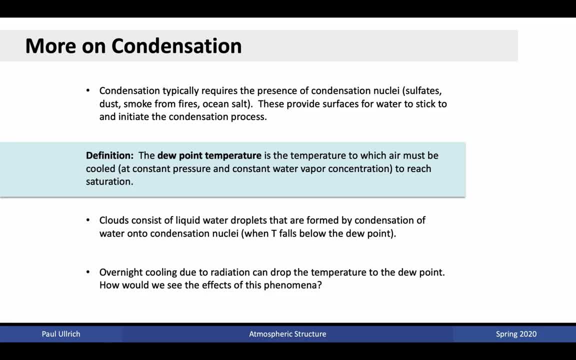 As temperatures drop, as air is lifted to higher altitudes, that air cools. When it hits the dew point temperature, which is the temperature to which air must be cooled in order to reach saturation, condensation begins to occur. This is then located at the cloud base. 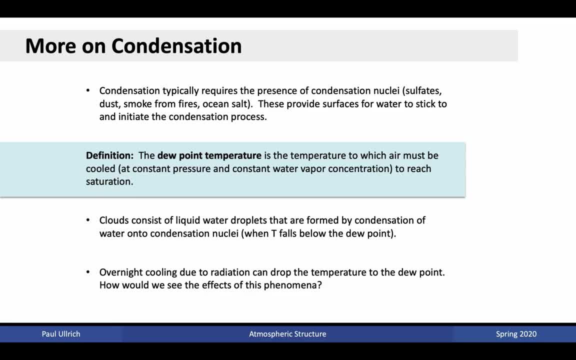 Above this point, where temperatures are even lower, one will then have cloud droplets occurring, and hence we will be able to actually visually spot the cloud in the atmosphere Overnight. cooling due to radiation can also drop the local temperature, And this is responsible for the formation of morning fog. 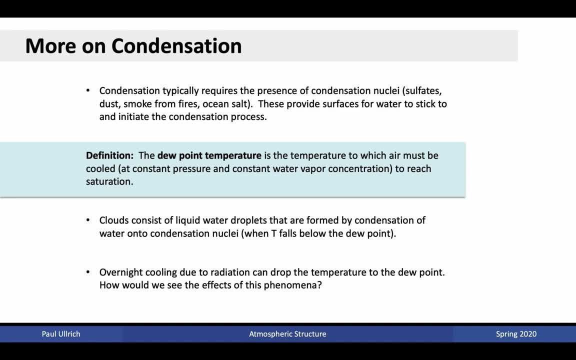 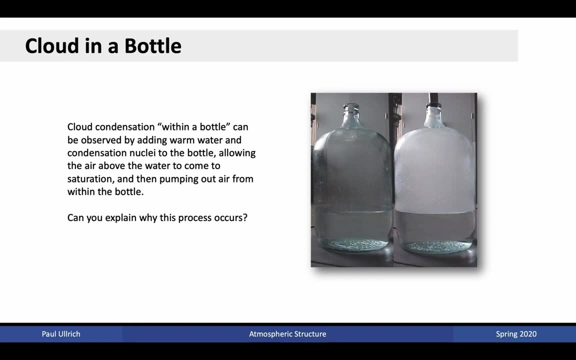 As temperatures drop overnight, the air cools and with that the water vapor that is present within the atmosphere may reach the saturation vapor pressure, leading to the formation of condensates. Cloud condensation can also be seen through simple cloud-in-a-bottle experiments. 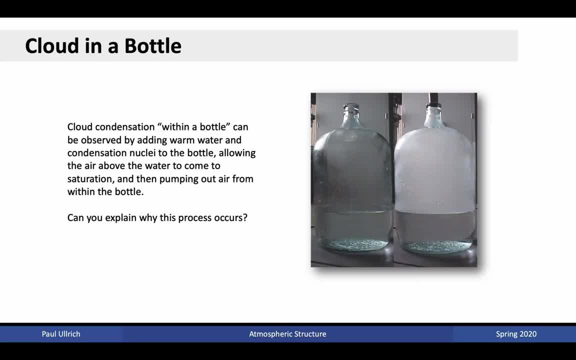 and I encourage you to Google YouTube in order to find some of these experiments that others have conducted. If one takes warm water, places it within a bottle, that air will quickly come to saturation. Recall saturation simply refers to water vapor molecules that are leaving the fluid at the same rate that they are entering. 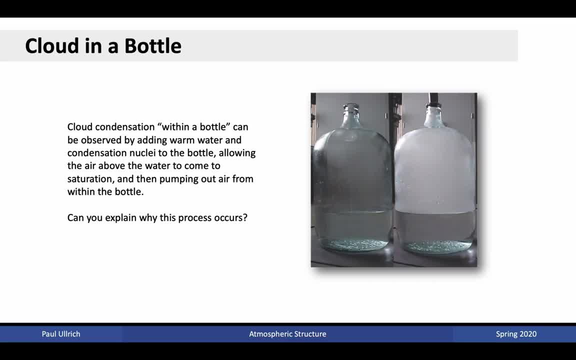 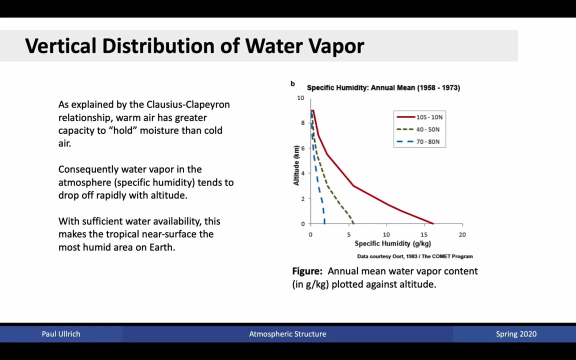 If we then pump some air out of the bottle and add smoke in order to provide condensates, one can then quickly observe, as the air cools, the formation of a cloud within the bottle. All right, By analyzing the information we have from the Clausius-Clapeyron relationship,